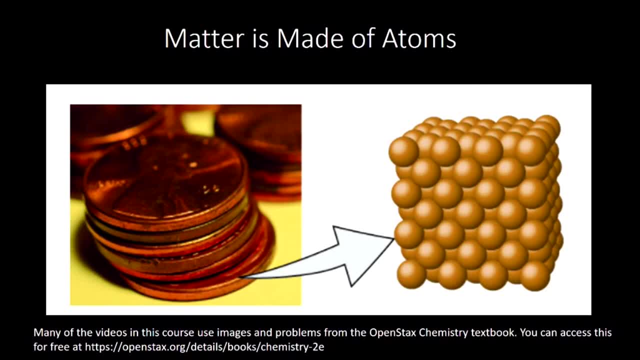 thinking about the smallest little piece of matter that you can't break apart, And the idea has been around since ancient India and ancient Greek thinkers suggested it. Now, what we call atoms and what they thought of as atoms aren't necessarily the same, but there's definitely a connection between this idea of a smallest little bit of matter. 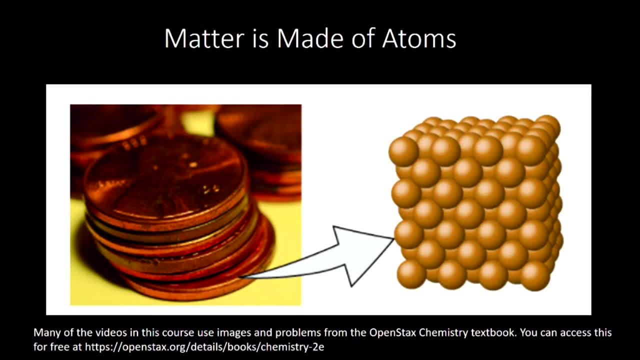 and what we now call atoms. Okay, so how did we start to think about the idea of atoms? Well, we started to think about the idea of atoms. We started to form a scientific idea of what atoms are like. We'll start with a scientist. 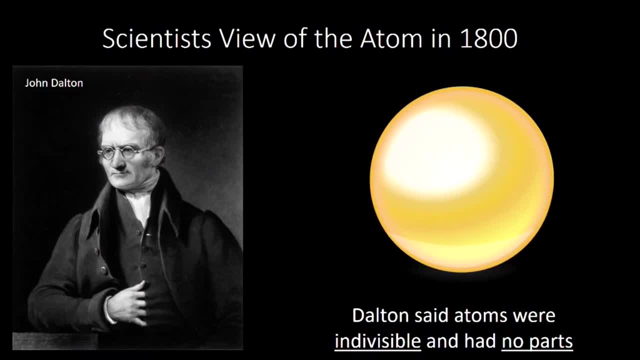 named John Dalton And in the 1800s he was the first one to use the Greek word adamos to talk about atoms in a scientific context. What did he say about atoms? Well, he said that they were indivisible and that they had no parts. So you can see here that golden sphere. 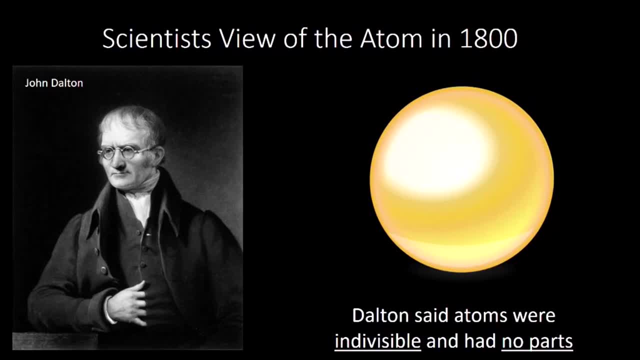 no parts, just a solid gold sphere. So imagine, for example, that you started with a gold block. right, You won't go, and you get a nice giant pure gold block and you cut it in half. Okay, no problems, You cut it in half again, and a half again and a. 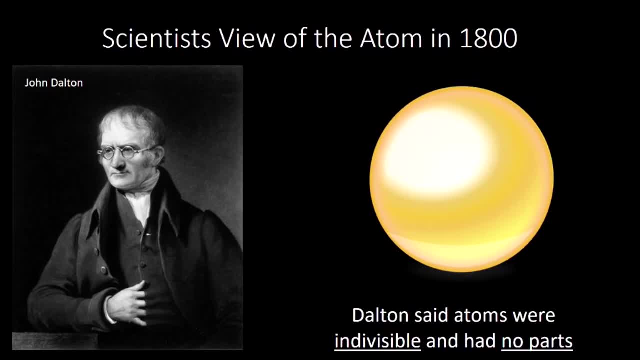 half again. The question is at the bottom of that: would there be a point where you could not cut it in half any longer, where there was the smallest little indivisible chunk of gold and you could go? no smaller? Dalton said: yeah, and that's an atom, It's the smallest little possible. 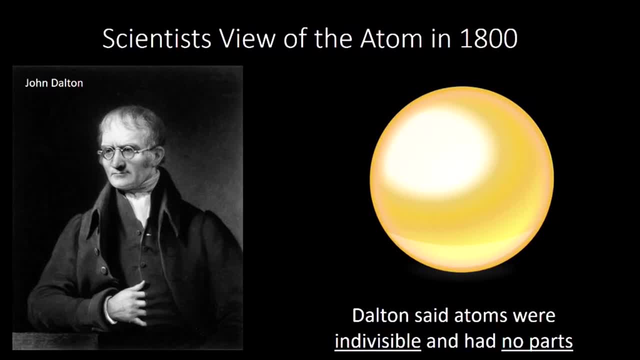 chunk of something we could have. It's just gold, but the smallest bit of gold, and it has no parts and it's indivisible. He actually drew representations of all of these different atoms, And here's his old school drawings. They're pretty cool, right, You can see. 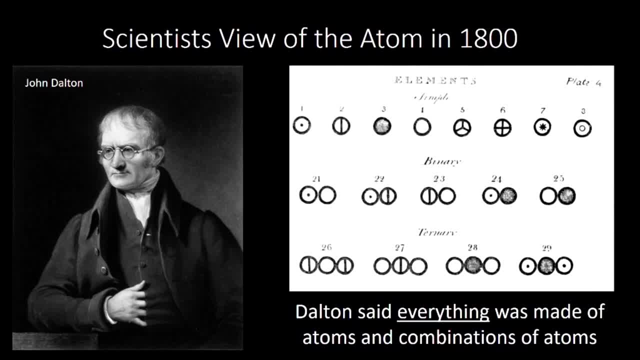 he said: okay, well, there's one atom type and he's going to represent it with a dot. So it's not as if he thought these were actually what atoms looked like, but he's just representing them in different ways. We use letters to do this. now He used shapes and 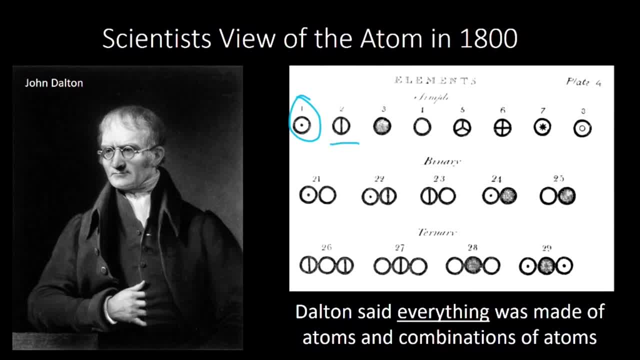 he said: we'll represent atom number two. It turns out to be helium, with this line And there's atom number three and atom number four. And he said: everything around us is made of these single atoms, but we can put them together. And he said: here you go, Here are some binary compounds. 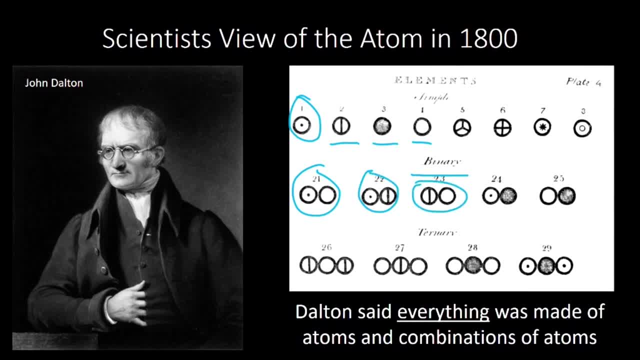 And these are made of two different atoms stuck together, And so this is a basic idea of atoms. That's the smallest little bits of matter, And then molecules would put atoms together, which is basically right. His picture of the atom left a lot to be desired, And we'll talk about. 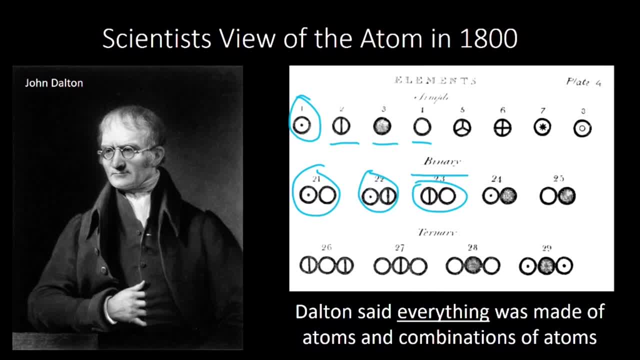 ways in which it was improved. but the basic idea that atoms are combined into molecules is totally right. It's totally right. Now, how did we advance from this picture of the atom? We no longer think of the atom as this solid chunk. How did that work? Well, 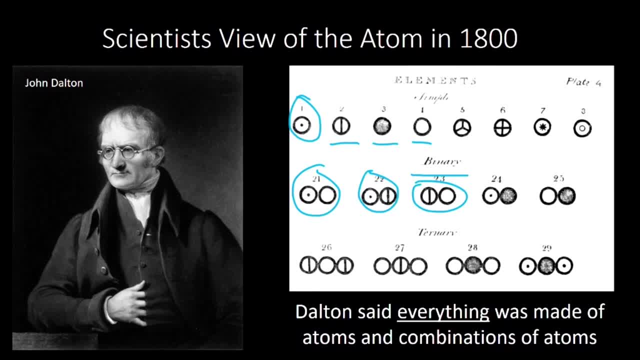 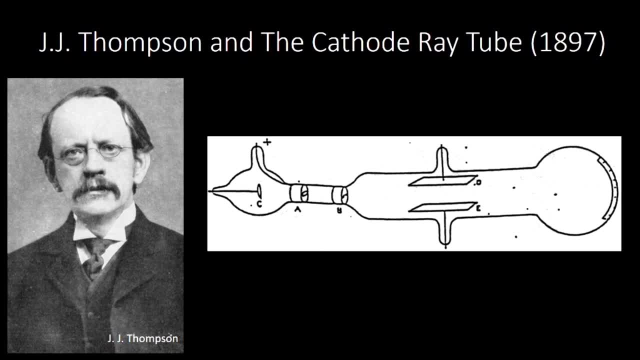 the first person to show with an experiment that atoms had parts was JJ Thompson, And JJ Thompson did this by studying something called cathode rays. And here we have drawn a cathode ray tube And I'll talk about the parts of it in just a second. JJ Thompson gave lectures. 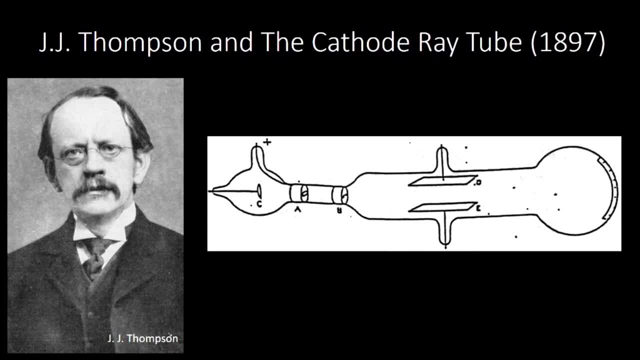 and gave demonstrations for the public. His wife Rose would often attend his lectures and demonstrations, which was actually unique for the time because women were only just recently allowed To watch these, which is crazy. So his wife would attend to all of them that she could. 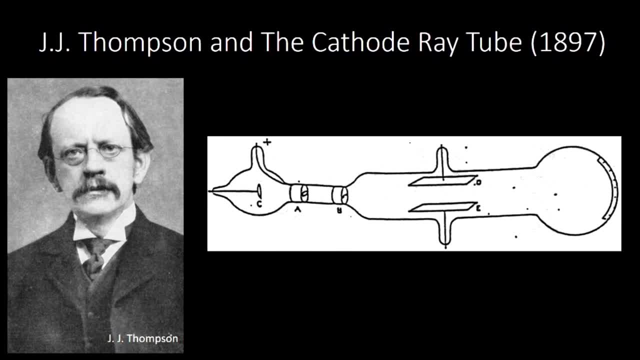 And so he showed with this cathode ray tube that atoms had parts. How do we do that? Well, first let's just talk about the different parts of this. It looks like kind of a complicated piece of equipment and we're going to simplify some, So we're just going to circle this whole. 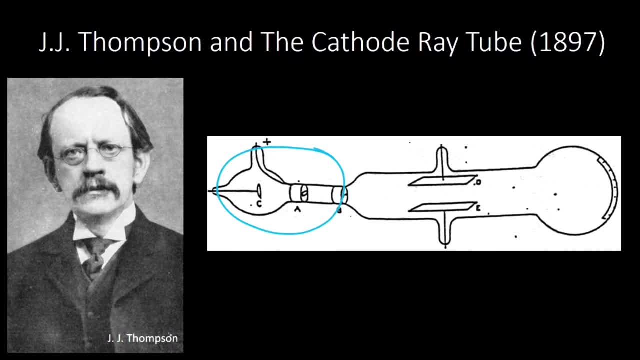 part and we'll just say that shoots cathode rays And that's basically what it's for. So that's like our cathode ray gun: It shoots cathode rays. Okay, So that shoots cathode rays, And then what happens is it goes down this pathway. 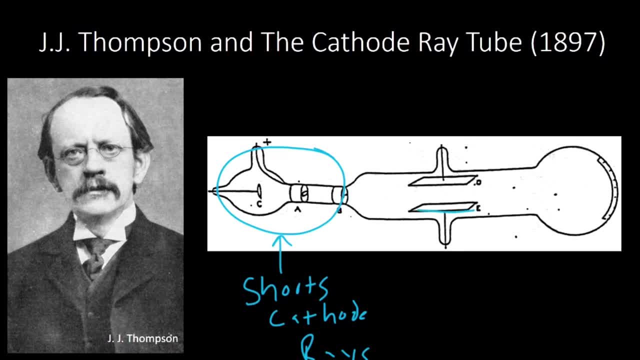 and what you see in D and E are charged plates. So those are charged plates. What it means to be charged is that they're basically connected to a battery. So maybe this one has a positive terminal of the battery and this one has the negative terminal of the battery. 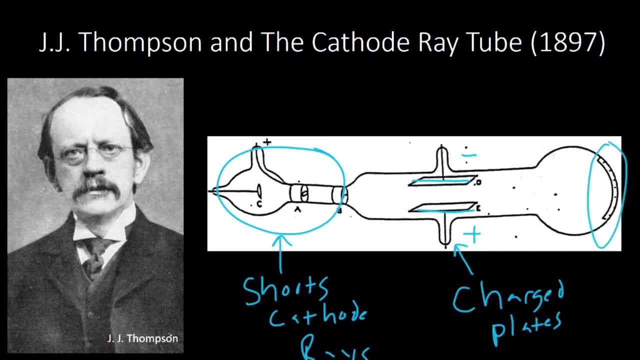 Okay, And then down here we just have this little screen and it's just going to detect where our cathode rays hit. In our video we'll actually just draw the cathode rays so you'll be able to see them. But in the real experiment we see where the cathode rays hit by looking at this little. 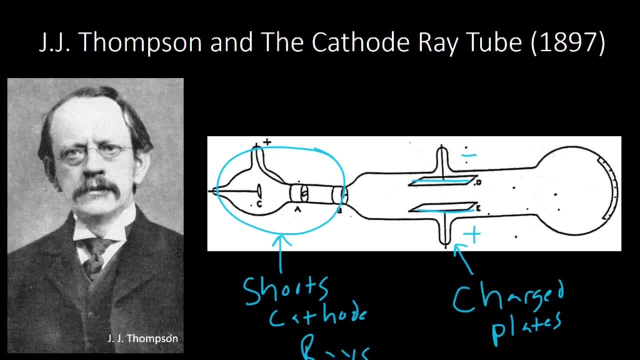 screen. All right. So what happens? Well, the cathode rays are shot down this pathway. All right, So we'll use grain and we'll say, hey, okay, the cathode rays are shot down. They pass through A and B. These turn out to accelerate the cathode ray And then it goes through these plates. 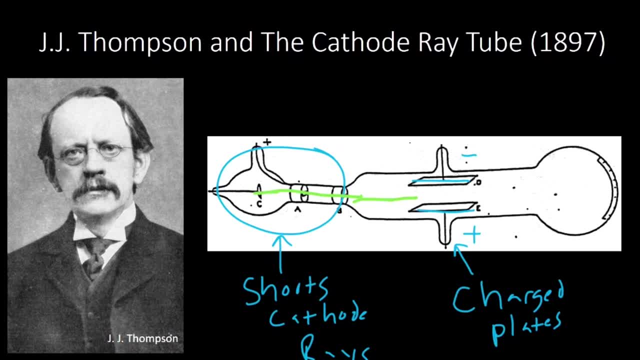 Well, here's what they noticed. What you might think is: oh, maybe it's going to go just straight through, But it didn't. Instead, it bent And it very specifically, if we had the negative plate up top would bend this way: Boom, Okay. So what's happening there? The cathode ray is bending down. 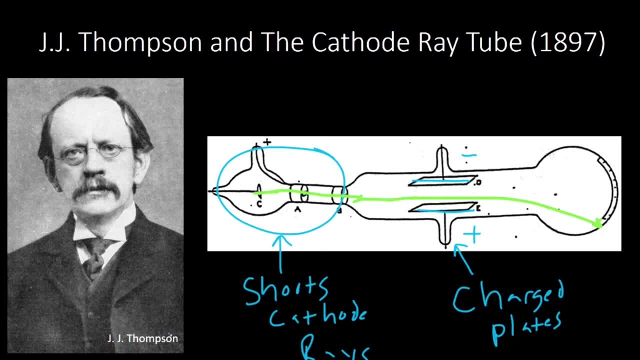 Why is it bent down? Well, it's being repelled by the negative charge on that top plate. Remember, we said: let's put a negative charge up there, Okay, And two negative things turn out to repel each other. And so, right from the start, they knew something in this cathode ray was negatively. 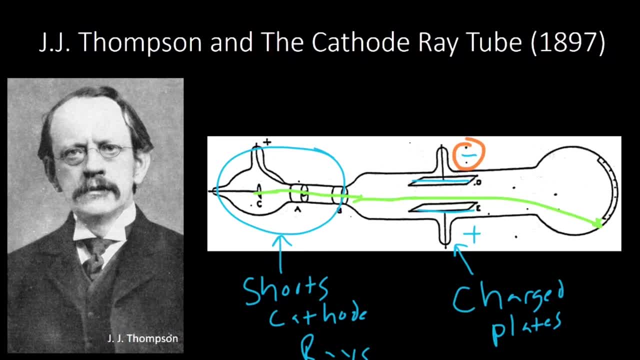 charged. Here's the cool thing: Based on how much it bent, they could actually calculate the mass of this thing. They could calculate how big it was. Okay, So we won't go into the details of that, But basically, if it bent more, it was smaller. If it bent less, it was bigger. Imagine, for example: 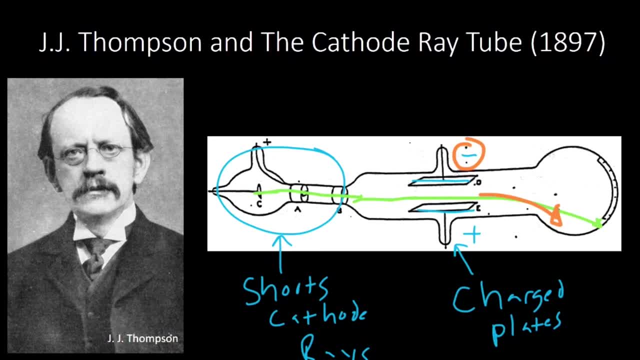 that you're driving a really big 18-wheeler truck. It's going 60 miles an hour And you try to turn it, It's going to turn more slowly. On the other hand, if you're driving a motorcycle, you can turn it really quick. So lighter things are easier to turn. Okay, And so based on how much it, 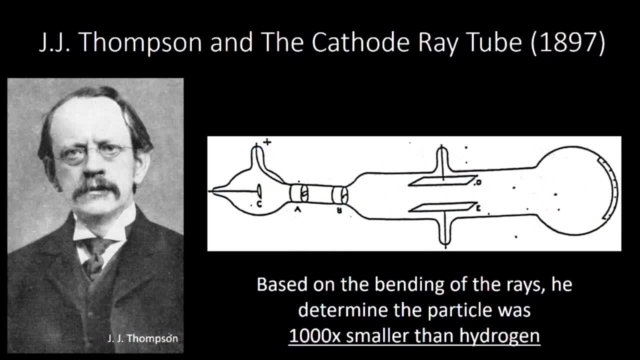 turned, we could tell what the mass was, And so, based on the bending of those rays, he actually figured out that the particle was a thousand times smaller than hydrogen. A thousand times smaller than hydrogen. Now, remember, Dalton had said the smallest element was hydrogen. And now JJ. 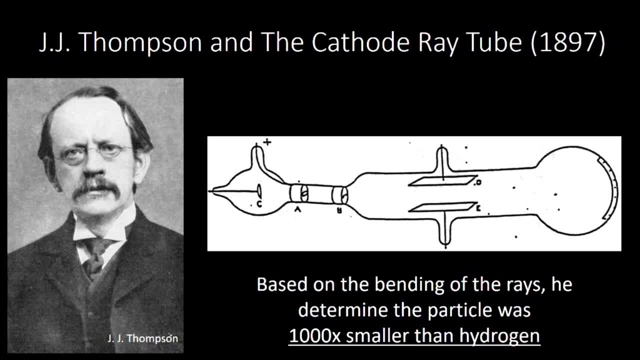 Thompson said: actually there's something way smaller. And if Dalton's claim that everything was made out of matter was right, that everything that was made out of atoms was right, then Thompson had just discovered that there was actually something that made up the atom A part of the. 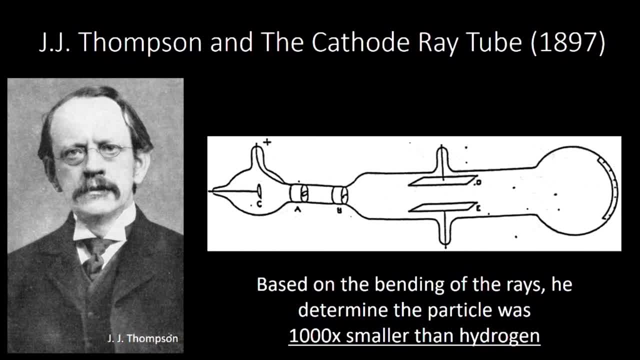 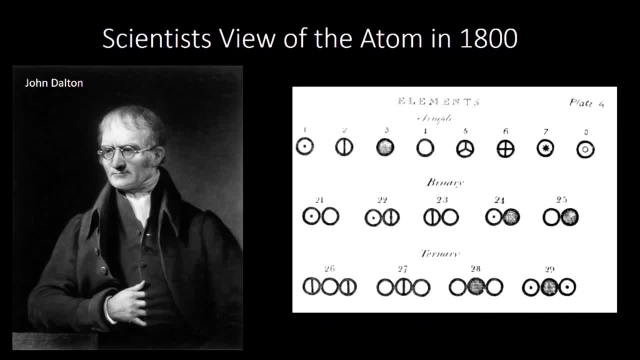 atom, Something that had fallen off the atom. The atom wasn't this indivisible, indestructible sphere, It had parts. It had parts. So here's Dalton, Our friend Dalton turned out that he wasn't quite right. What happened is one of his atoms lost something, And maybe this made Dalton 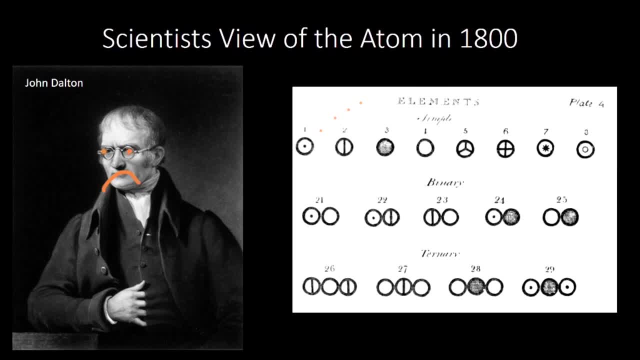